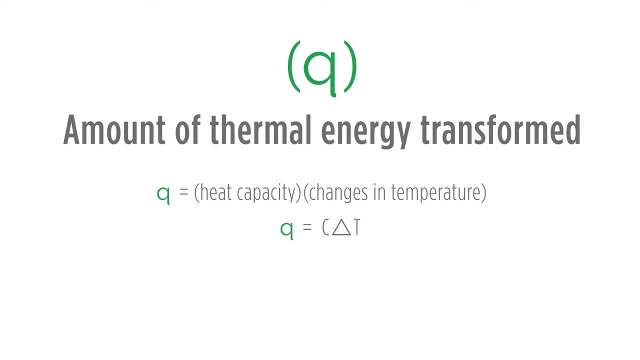 or symbolically, Q equals C delta T. For specific heat, the thermal energy transferred is equal to the mass times, the specific heat times, the change in temperature. Symbolically, Q equals M S delta T. The other thing we need to be aware of when we look at calorimetry problems is there's actually two bases. 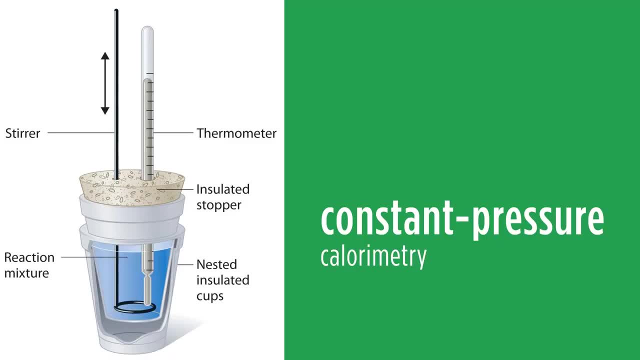 One is the basic calorimetry-type problems, one with constant pressure. Constant pressure calorimetry is very common and can be done with a simple coffee cup-type calorimeter. Constant volume calorimetry requires a specific type of calorimeter, a BOM. 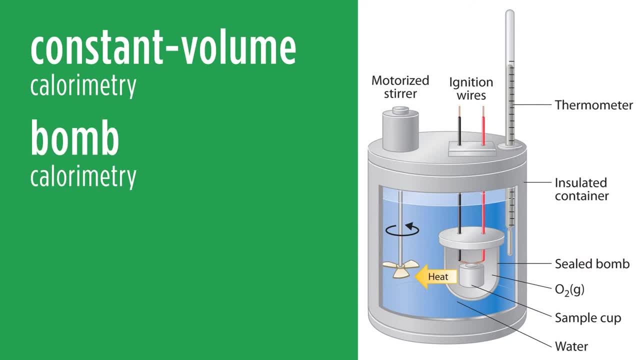 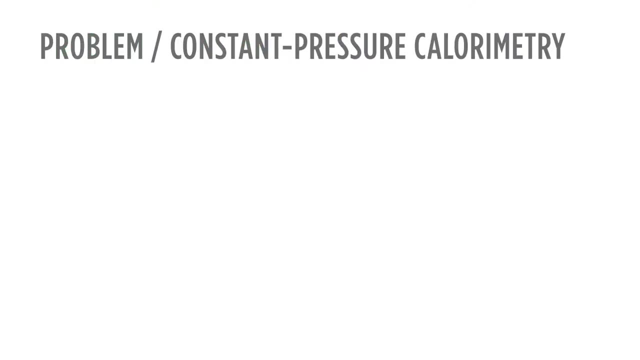 Therefore it's often called BOM calorimetry. First we're going to look at an example problem looking at using constant pressure calorimetry. Then we'll look at a constant volume calorimetry problem. Then we'll look at a constant volume calorimetry problem. 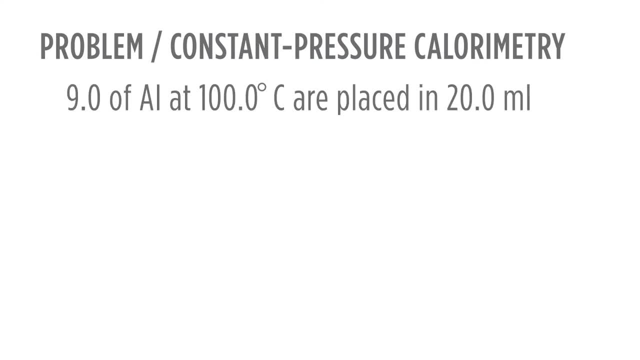 The problem: 9.0 grams of aluminum at 100 degrees Celsius are placed in 20 milliliters of water at 20 degrees Celsius, contained in a coffee cup calorimeter. At thermal equilibrium, the temperature of the water and the aluminum is 27.1 degrees Celsius. 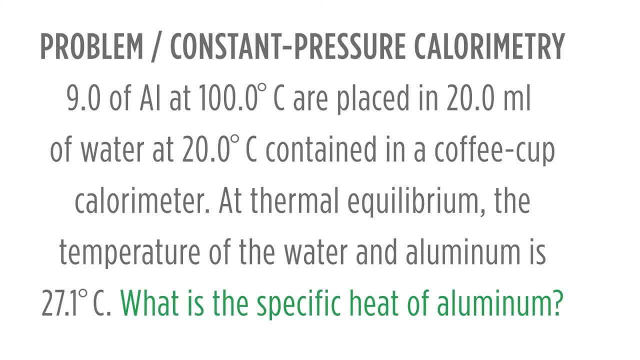 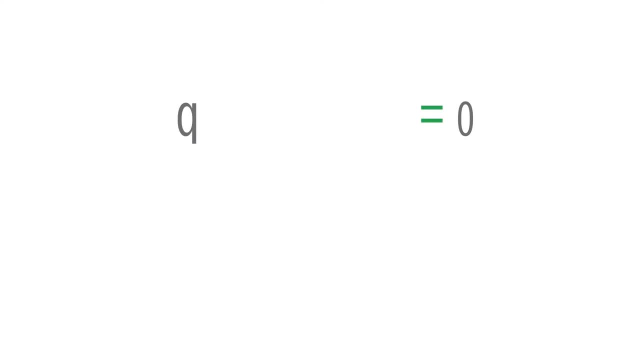 What is the specific heat of aluminum? Again, remember that the thermal heat transferred, Q, will be equal to zero. and here we have the heat transferred, Q for aluminum transferred into the calorimeter Q-cal. So therefore, Q for the aluminum is equal to negative Q for the calorimeter. 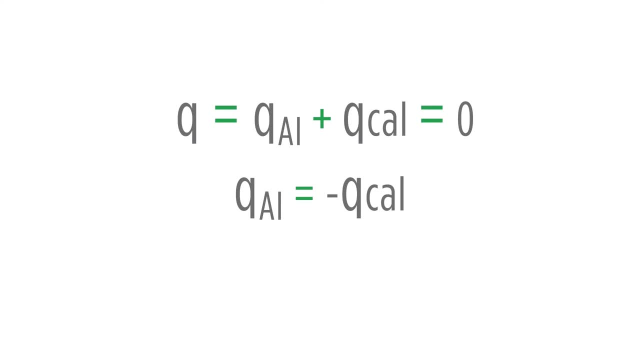 Since we've been given the specific heats for these, or we're actually looking for the specific heat, we can use the specific heat formulas. So Q equals M-S-delta-T. If we substitute those in, we'll see that we have M-aluminum. 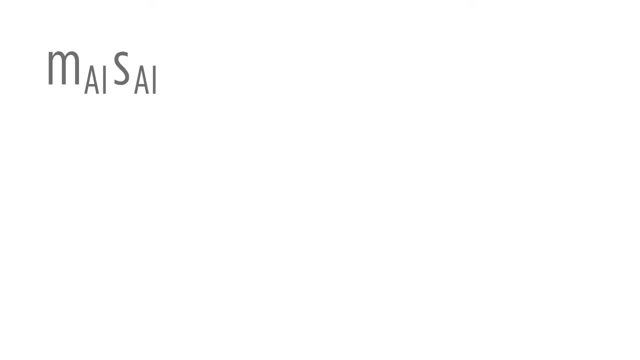 aluminum: specific heat- aluminum. change in temperature for aluminum is equal to the negative of the mass of water times the specific heat of water times. the change in temperature of water- If we do a little algebra we get specific heat of aluminum- by itself is equal to negative mass of water. 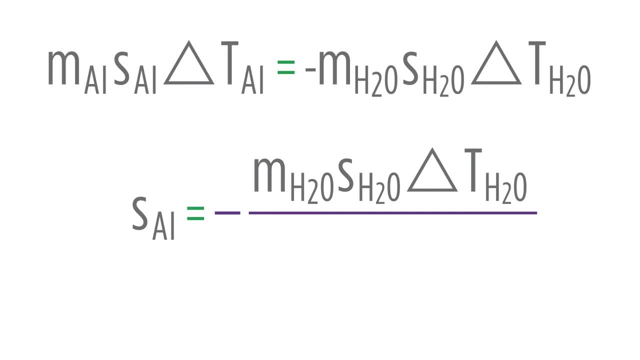 times the specific heat of water, times the change in temperature of water over the mass of aluminum. times the change in temperature for aluminum. If we look at the values we need and the problem, we can come up with some of these very quickly. Mass of aluminum is going to be 9.0 grams. 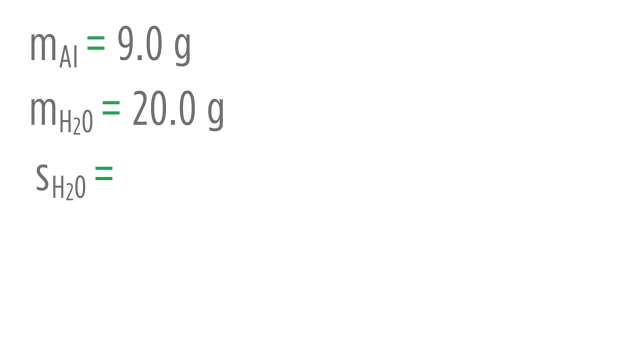 Mass of water is going to be 20.0 grams. The specific heat of water is 4.184 joules per gram degrees Celsius. For temperature, we know that the change in temperature is equal to the temperature final minus the temperature initial. 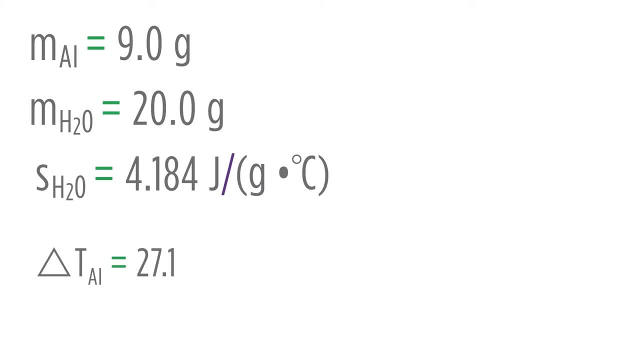 Therefore, the delta-T for aluminum will be 26.5.. 27.1 minus 100 degrees Celsius, which is negative 72.9 degrees Celsius For the change in temperature of water, we have the final temperature 27.1 minus the. 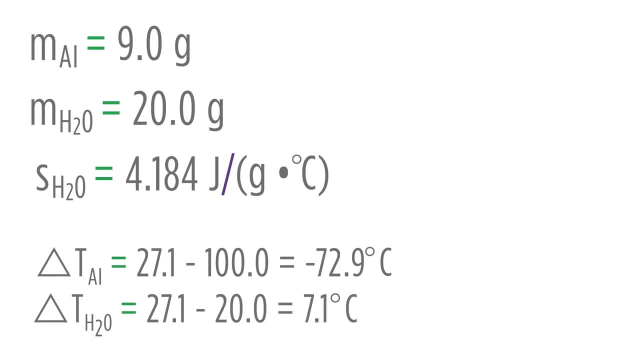 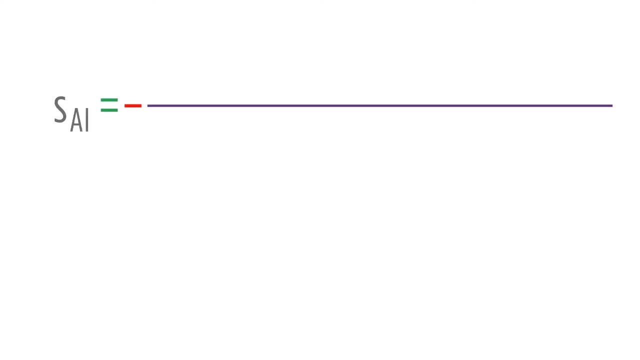 initial temperature 20.0, which gives us 7.1 degrees Celsius. Plugging this all in, we get the specific heat of aluminum is equal to negative 20.0 grams multiplied by 4.184 joules per gram per Celsius, times 7.1 degrees Celsius divided. 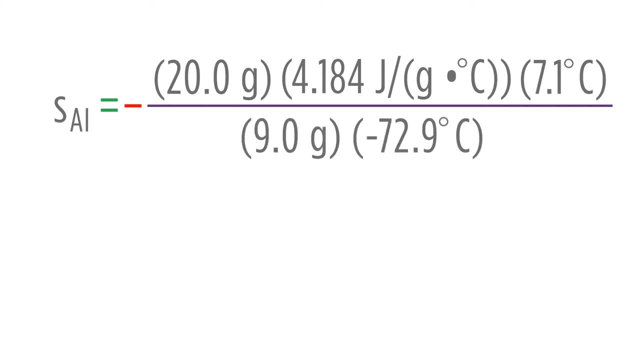 by 9.0 grams times negative 72.9 degrees Celsius. We can see that on the top of our formula the grams cancel out and the Celsius cancel out, leaving us just joules. When we do our calculation, we see the specific heat of aluminum is: 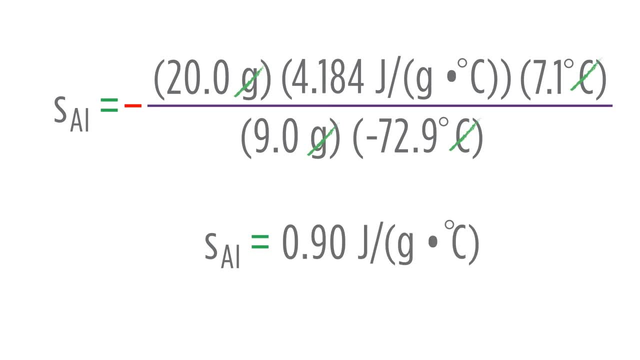 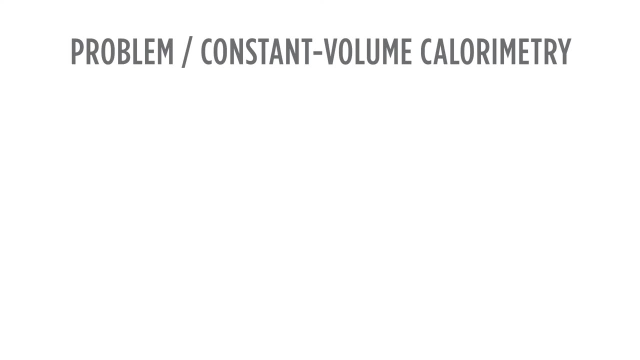 equal to 0.90 joules per gram degrees Celsius. For the constant volume calorimetry problem, we're going to look at a combustion problem. This is very common for constant volume type calorimetry or bomb calorimetry problems. Combustion of 1.00 grams of sucrose causes the temperature of a bomb calorimeter. 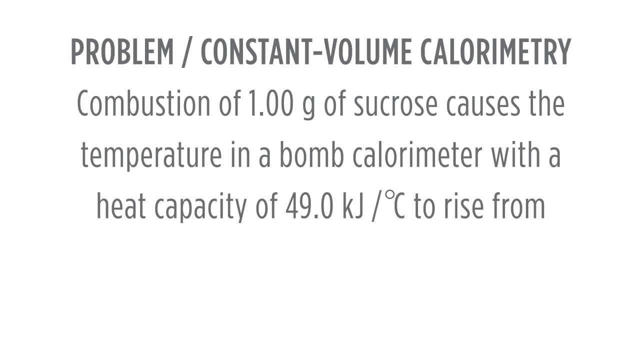 with a heat capacity of 4.90 kilojoules per gram. In this problem we see that we have a bomb calorimeter and they're giving us the heat capacity of the bomb calorimeter. Therefore, we're going to use the Q equals heat capacity. times: change in temperature.